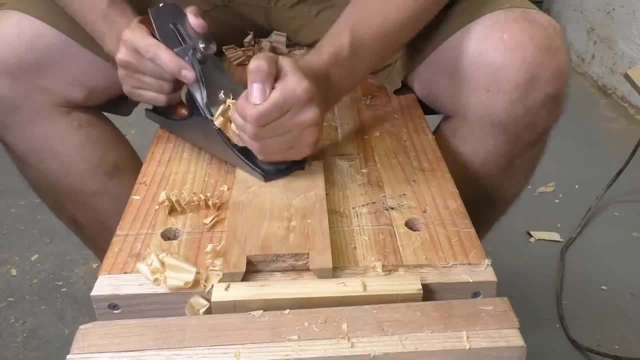 with the plane. I did the outside of all the boards, which is okay, but I also did the inside of all the boards, which is okay. but I also did the inside of all the boards, which is okay- inside of one of the boards and that was really stupid of me because planing the inside surface. 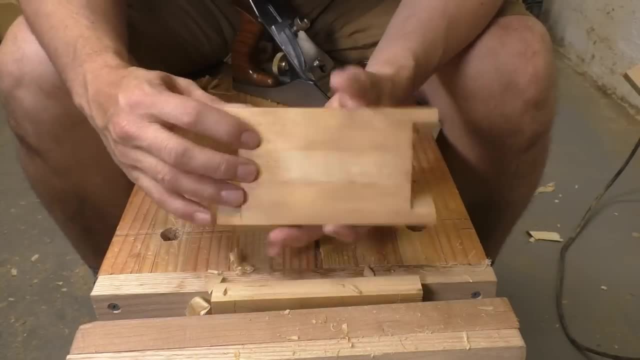 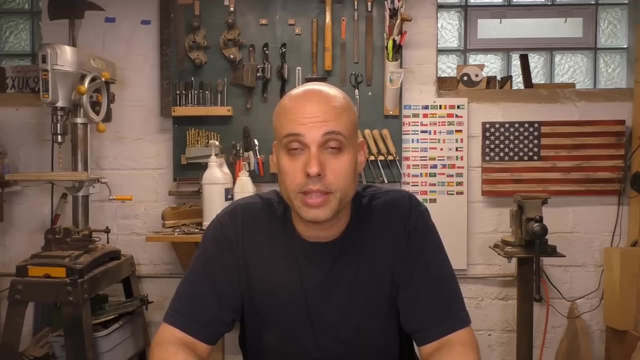 can mess up your joint and give you gappy, awkward shoulders. Luckily, I only did this to one of the boards, so it is a totally recoverable mistake. But be smarter than me. If you're going to finish planing the boards, stick to the outside or just wait until after glue-up, when it'll be safe. 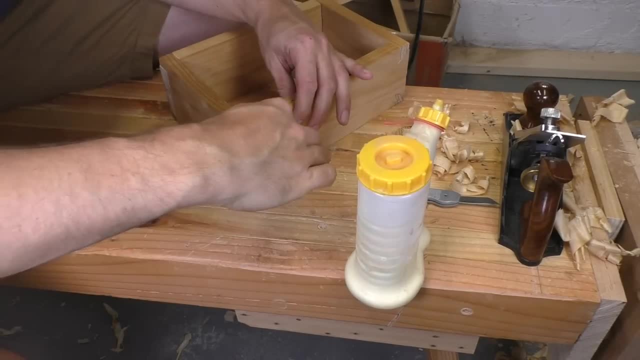 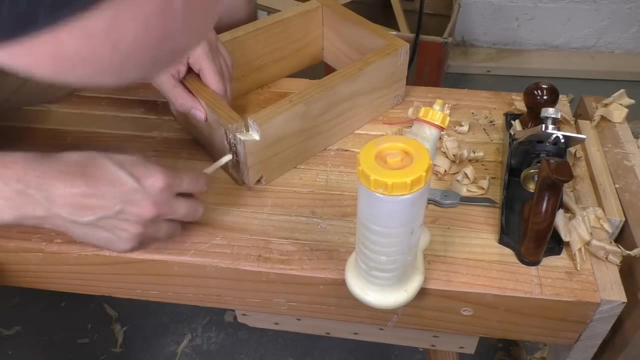 For gluing these joints up you only need a little bit of glue. Dovetails, even mediocre ones, hold themselves together pretty well with no glue at all. So you want to concentrate on the long grain surfaces and just put a little bit of glue on the end grain. 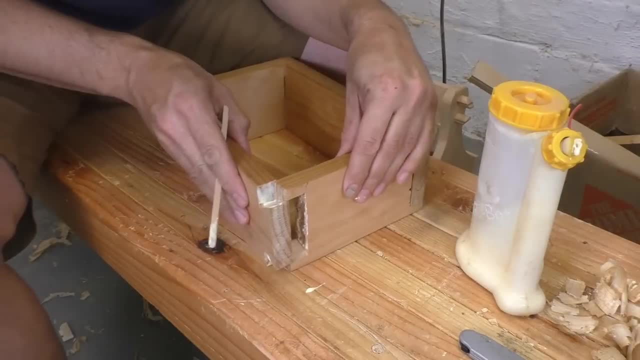 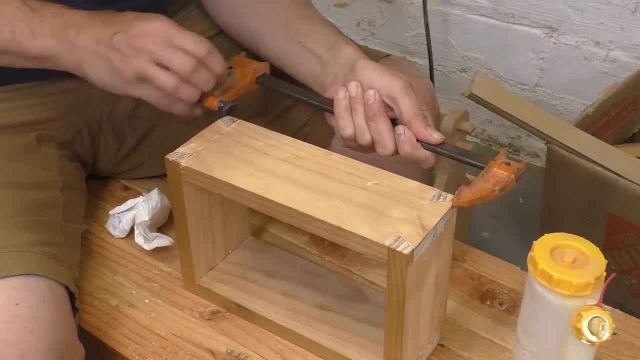 This is mostly to hide gaps. The end grain doesn't have a lot of holding power. Now, a really good dovetail hardly needs any clamps at all. but my dovetails are only okay and the clamps are going to allow me to put a bit of pressure on the joints and close up a lot of the 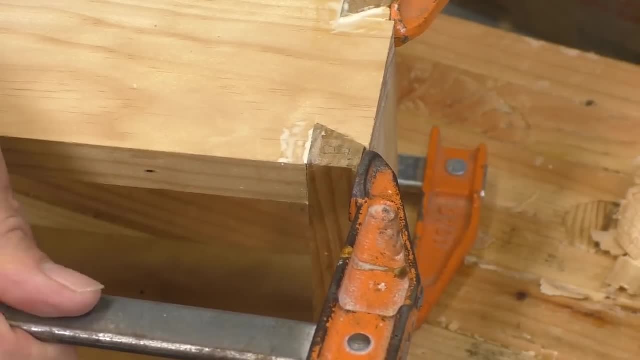 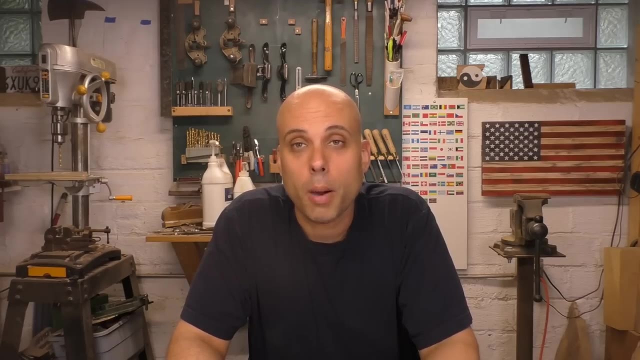 little gaps, I have Too much pressure and you'll snap your pins. but just a little bit of clamping pressure hides many sins. If you find you have gaps that the clamps can't comfortably squeeze shut, don't try too hard. We cut all those slivers of wood and we can use those to. 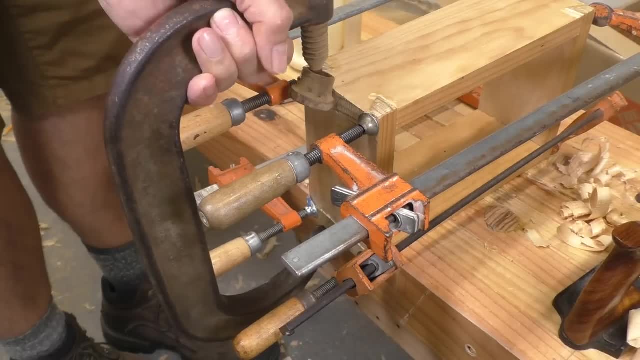 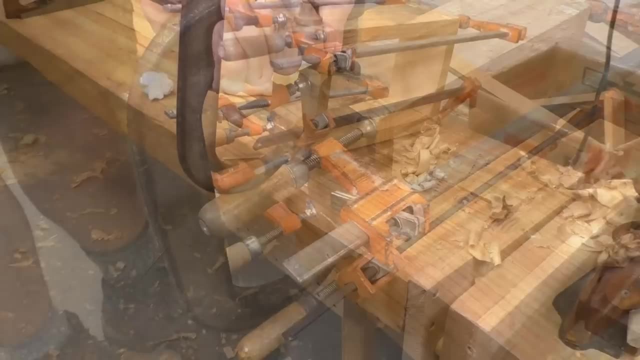 fill up any problem areas after the glue dries. As you're gluing and clamping, you might find that your board also needs a little pressure on the tails, and a nice C-clamp is really useful for that. When I'm all done with the clamping, my box looks a little bit like a porcupine with all these. 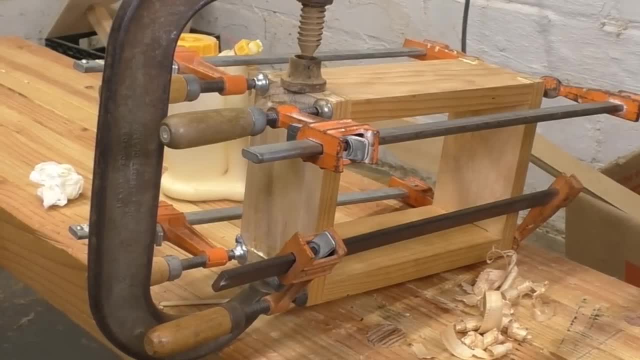 things sticking off of it. but future boxes aren't going to need this treatment because my joints will get better and they'll need a lot less clamping during glue-up And once the dovetailed box comes out of the clamps, any little bit of clamping will be enough to hold the board in place. 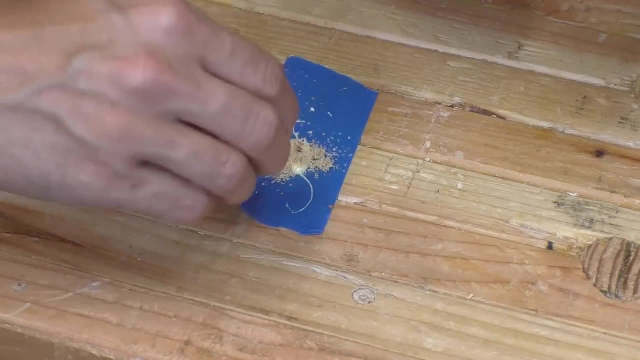 And once the dovetail box comes out of the clamps, any little bit of clamping will be enough to hold the board in place. Any little remaining gaps I didn't fill in with wood chips can be filled with a quick mixture of glue and sawdust. Once that's sanded flush, it'll be surprisingly invisible. 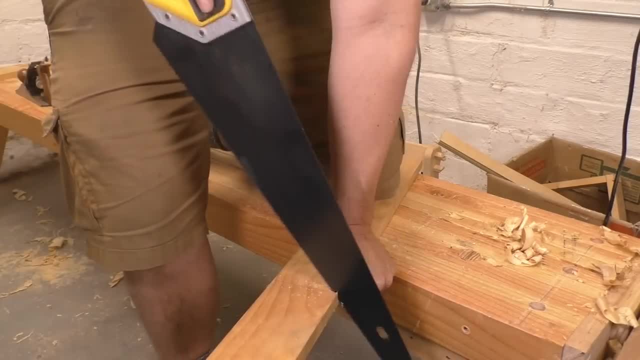 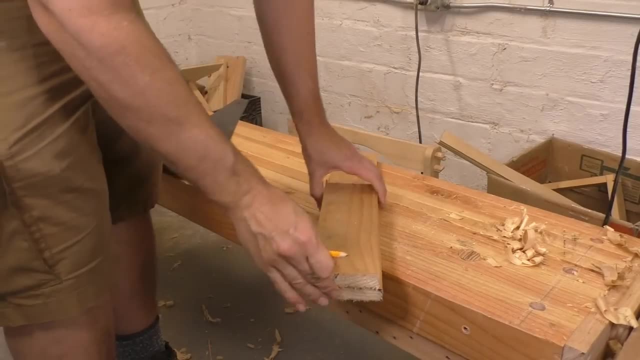 While the box assembly dries, I'm going to work on the top and the bottom, Just like in our last video. I prepare my components with fast cross cuts and I mark all the components from the first one I cut. That means they're all going to be the same size. with no measuring, I chose good. 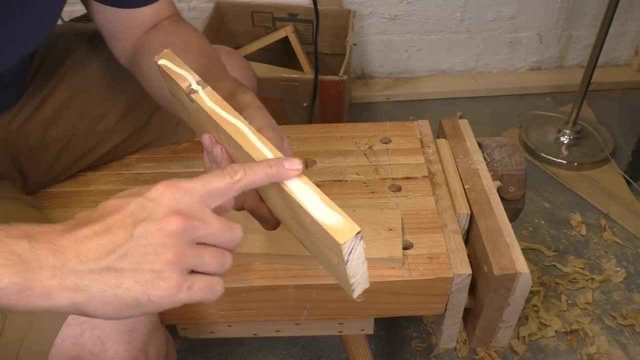 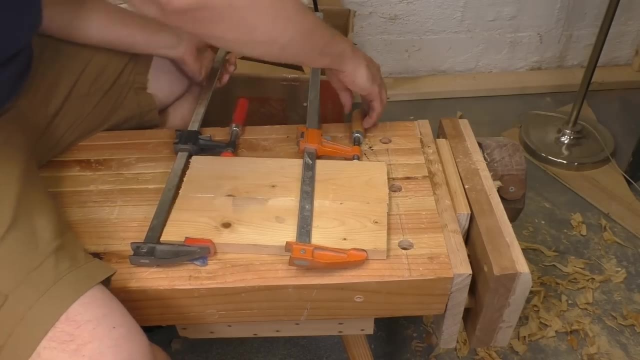 straight boards for this project, and so there's no need to joint the edges. I just glue them and clamp them up and I'm going to get a clean joint. I use my best cleanest boards for the top and any old scrap wood for the bottom. Nobody really. 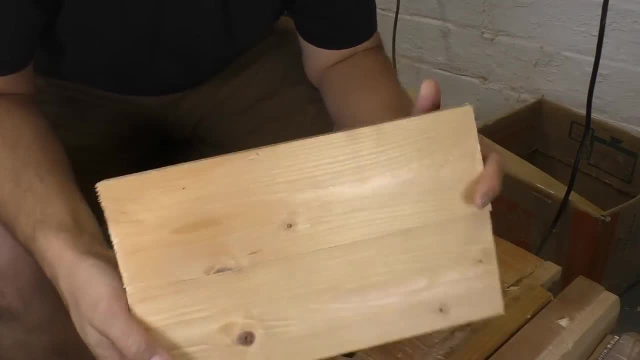 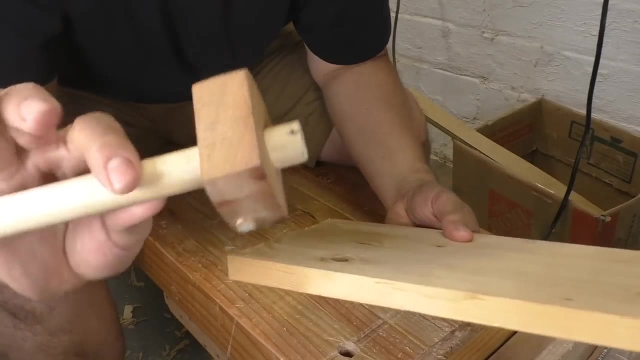 pays attention to box bottoms. Both my top and bottom come out of the clamps looking great, but they're too thick and chunky. If I leave them like this, the box is going to be awkward looking and clumsy. So I want them to be thinner, to give the box a little bit more of an 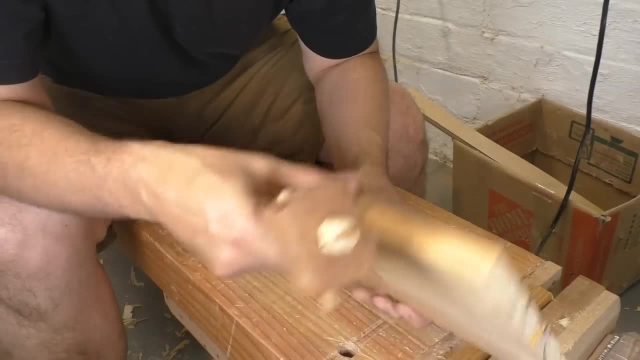 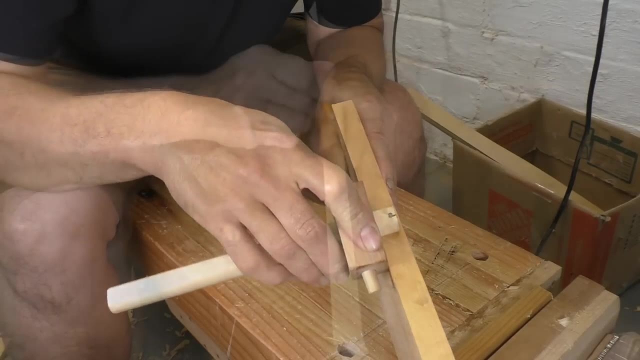 elegant look overall. This is a great time to practice dimensioning stock by hand. People think this is a huge headache, but it's really not bad at all. You'll want to gauge a half inch depth line all the way around the board and darken it in with a pencil to make it easy to see. 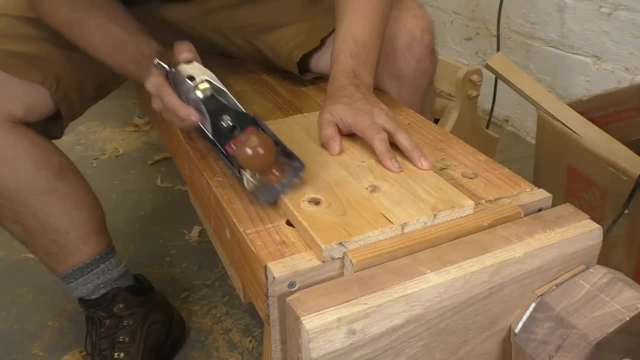 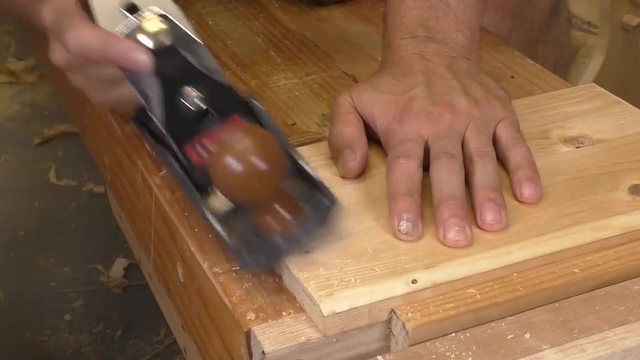 Then you can take your scrub plane and plane a bevel down to these lines. That gives you an easy visual reference all around the board And with everything beveled down to the gauge lines, all you have to do is plane off the waste in between those bevels. We're going to start out. 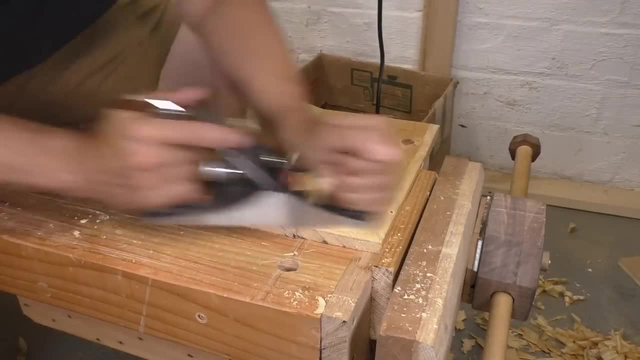 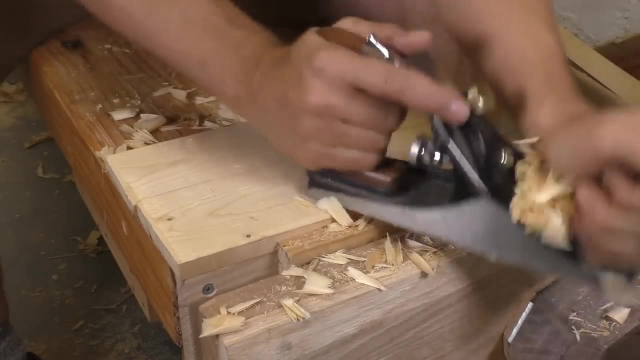 by traversing, which is a fancy way of saying we're going to go across the board. This gives us quick removal of material with minimal tear out, And when I'm close to my lines I'm going to flip the board lengthwise. keep my scrub plane and go with the grain When your bevels disappear. 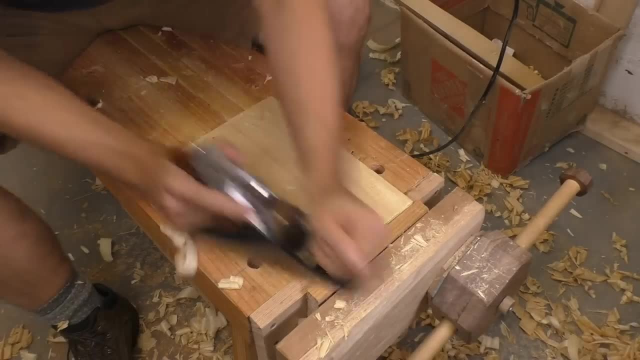 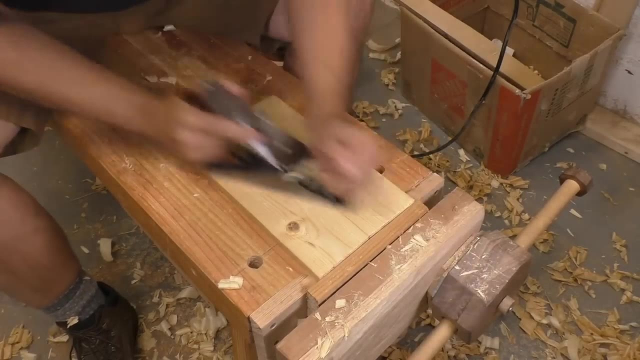 you can switch to your smoothing plane. I'm using my Grizzly plane here. I reviewed this two weeks ago as part of my all summer long hunt for the best affordable smoother. You can watch that video and I'll have a couple more plane reviews before the summer is over. Using a finely set smoothing. 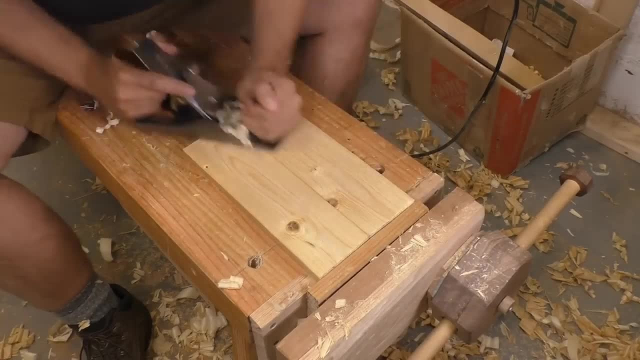 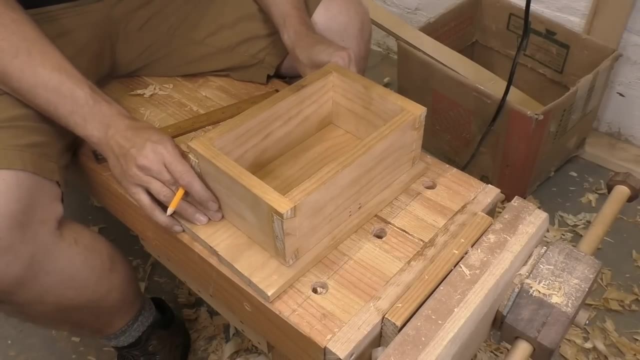 plane like this allows me to get right down to my lines and end up with a flat, nice finish with no tear out. When I was doing the glue up for my top and bottom of my box, I left these pieces long intentionally. That gives me wiggle room later on to fit them to whatever I 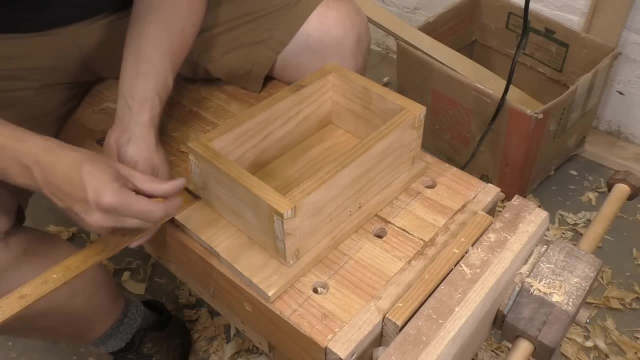 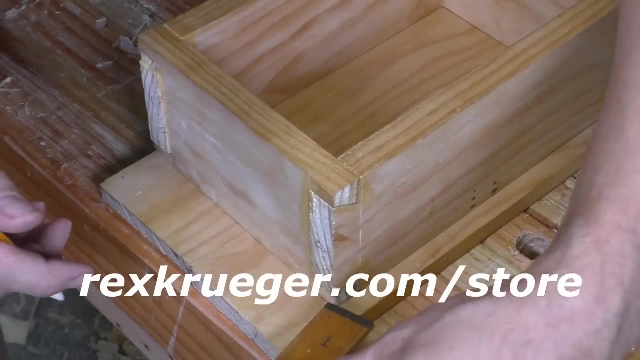 want, I'll set my box on the lid or the bottom and give myself a nice overhang all the way around. All the exact measurements are in the plans and you can grab those at rexkrugercom slash store or click the link down in the description. All my plans are super affordable. 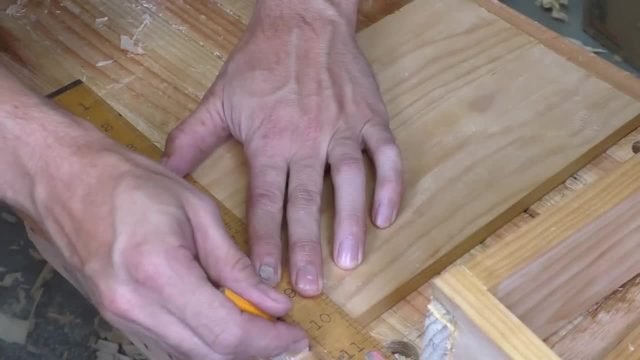 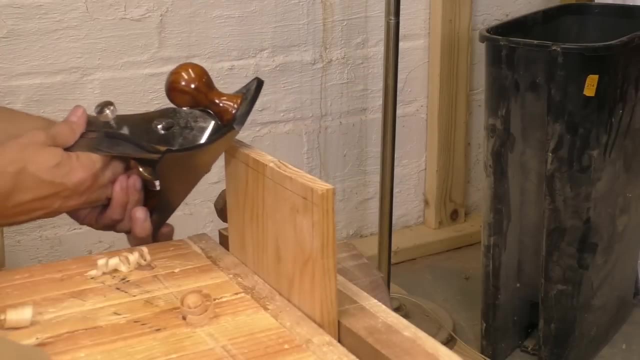 After I like the margins on my top and bottom, I'll strike my line cross, cut my waist and shoot everything square on my shooting board. Now I want to put round overs on my top and bottom. This is going to give a nice finished look and add a lot of chip resistance to those sharp edges. 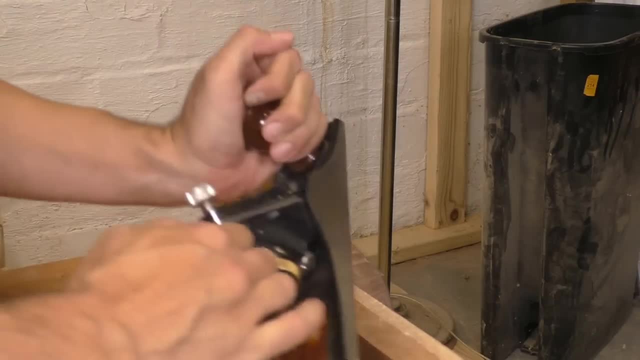 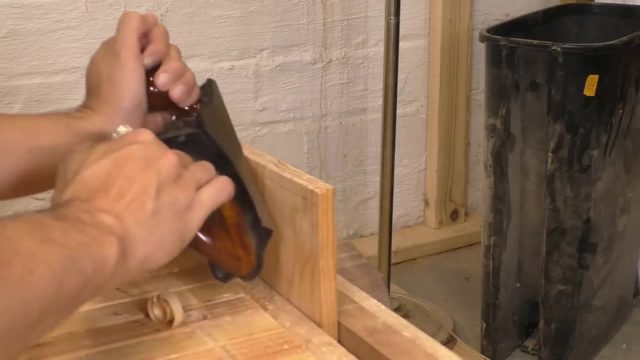 especially using a soft wood like pine. You might think you need a router to cut nice round over details, but you can do a great job with just a hand plane and a little sandpaper. I'm going to start by doing my round over details on the ends of my boards because 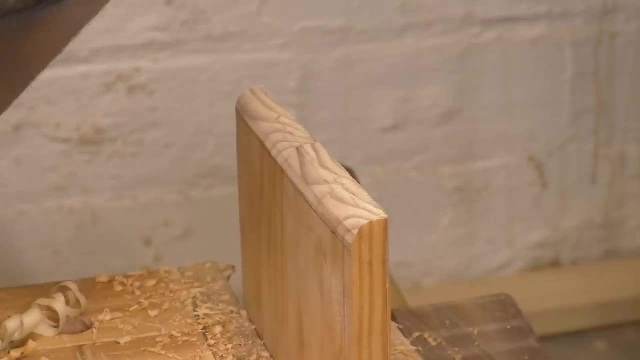 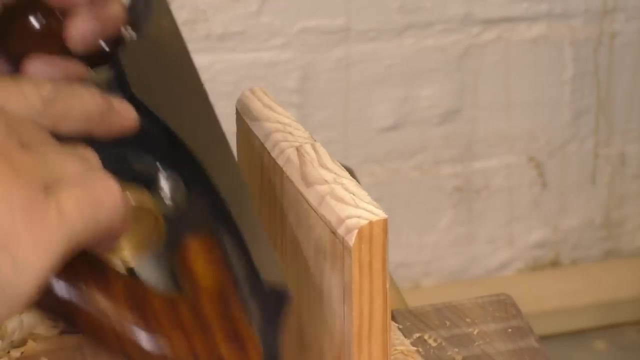 these are the most likely to blow out. while I'm planing, I'll nip a little bevel on the far end and skew the plane. I'll plane my round over in with a slightly circular motion and judge the shape by eye. It's all you need to get a clean curve. 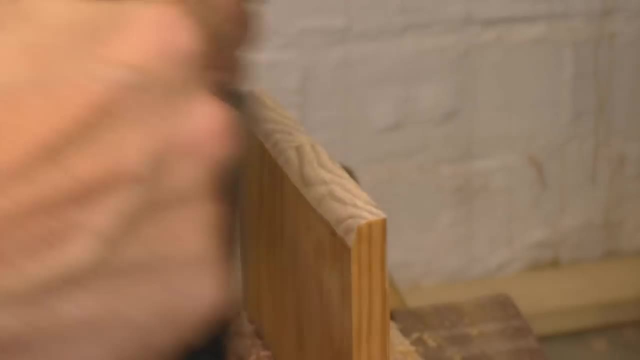 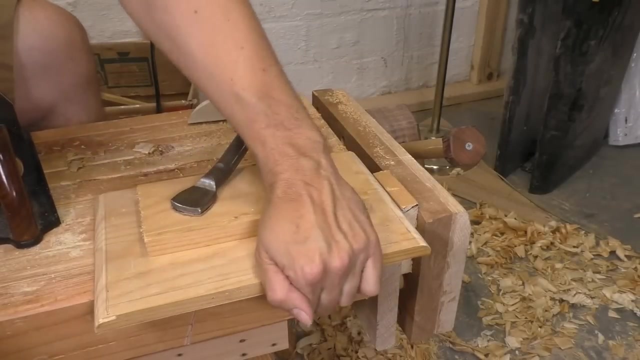 Then I'll flip the board around, do the opposite end and just make them match by looking at them. You can do a great job just with your eyeballs. I didn't get any blowout while I was doing these round overs, but if it does happen, leaving the long grain edge for last will allow you. 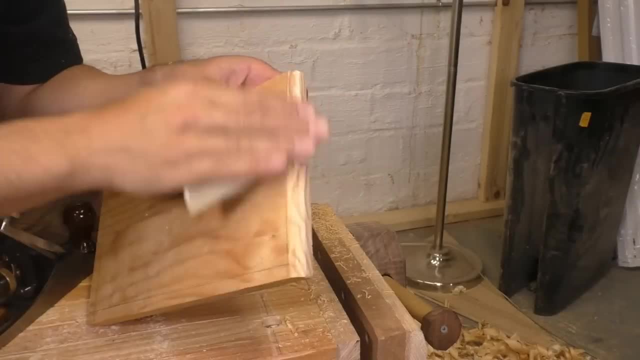 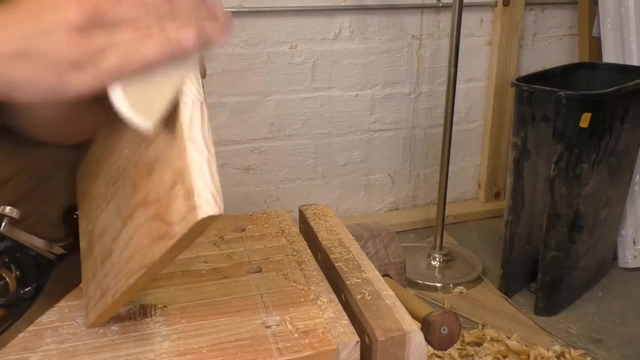 to plane any damage away very easily. Once your bevels are finished, you can sand them with some 180 grit sandpaper, and sand them with some 180 grit sandpaper, and sand them with some 180 grit sandpaper, And they come out looking great, just as nice as anything I've ever done with a machine tool. 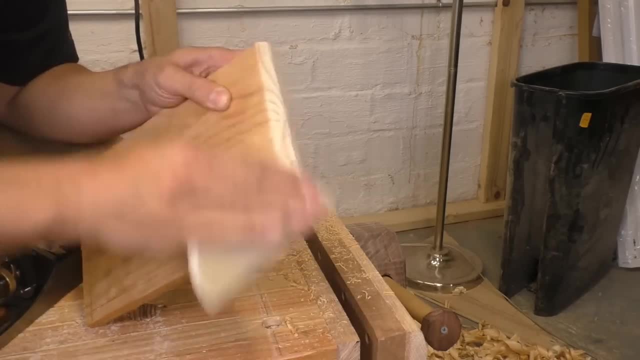 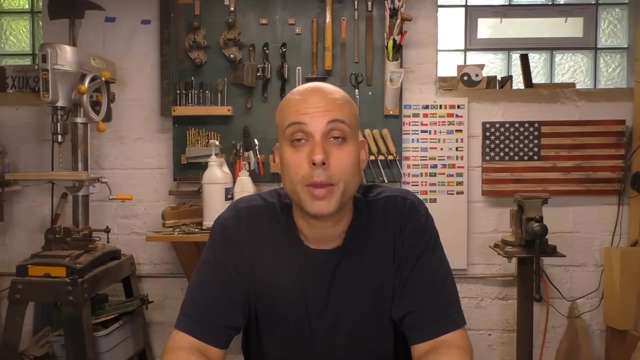 This box is simple and the top and bottom are exactly the same, So just plane the bevels to match on both pieces and you're done. Now we're in the home stretch of our project. All the components are made and we're ready for assembly. I've intentionally left the 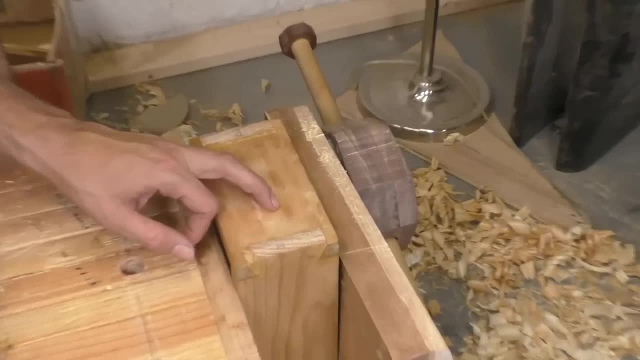 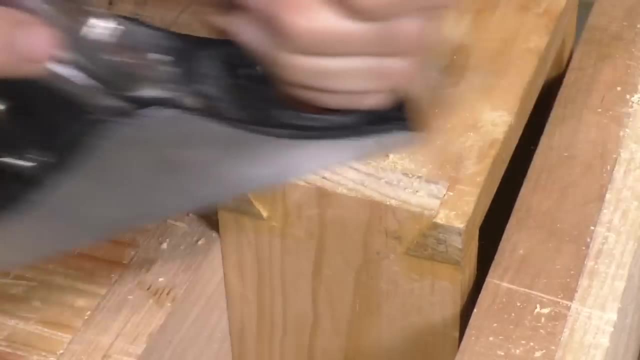 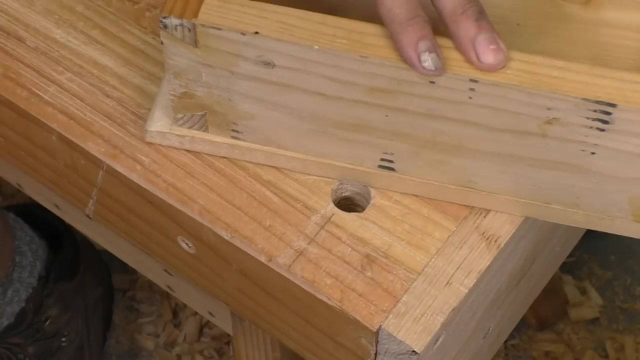 joints on my dovetails a little bit proud and they need to be planed down. You'll want a sharp iron and a fine set to your plane. Go slowly and creep up on a final flush surface. At this point I notice that my box is not exactly square, so my top and bottom look a little odd. 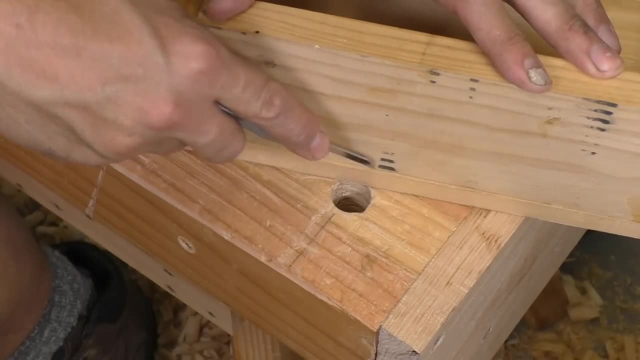 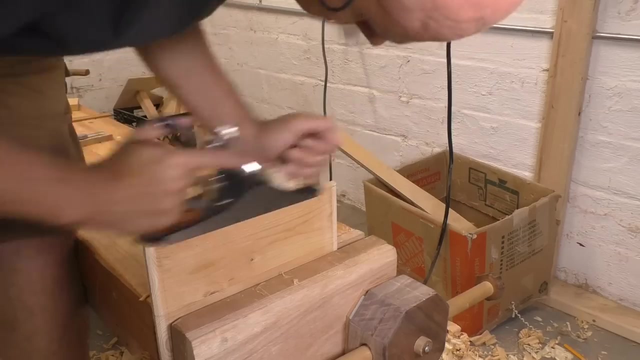 This is no big deal. I'm just gonna trace the out of square edge onto my top and bottom pieces and plane them down to match the box frame. No one will ever notice. And then, especially because this project is pine and it's a little bit soft, it's gotten very. 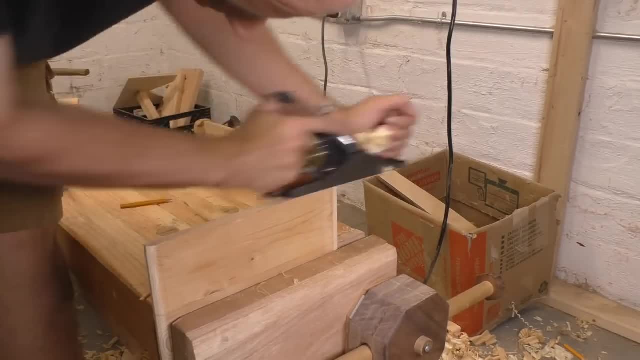 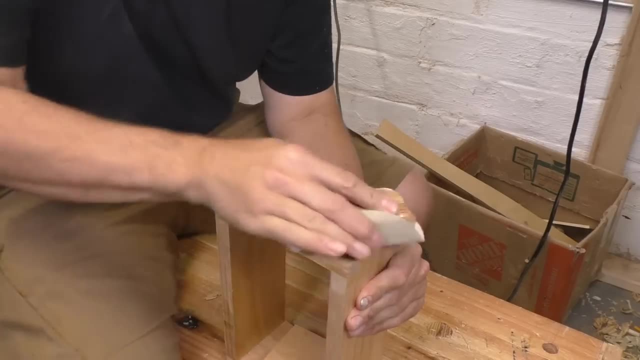 dinged up from the whole assembly process. The whole thing benefits from a nice light sanding. You can wrap a piece of sandpaper around a block to keep everything straight. straight and square, and I did a little bit of it that way, but then I just broke out. 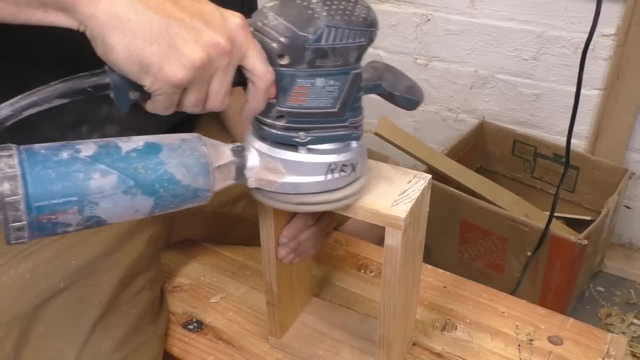 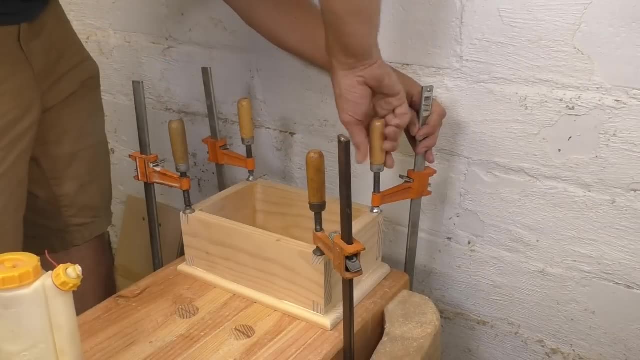 the random orbital sander to speed things up. Sanding this project gives it a nice clean finished look And once all the parts are surfaced I can glue on the bottom and clamp it. You can finish off a box like this with some super cheap hinges. 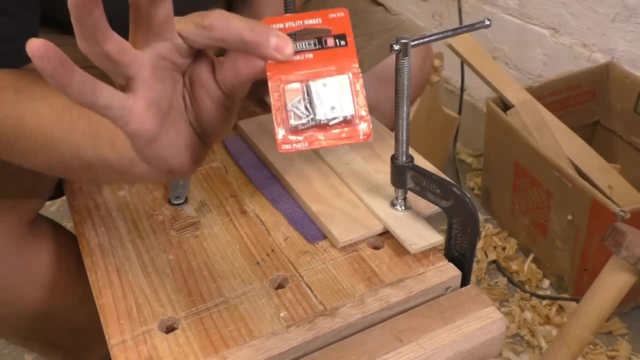 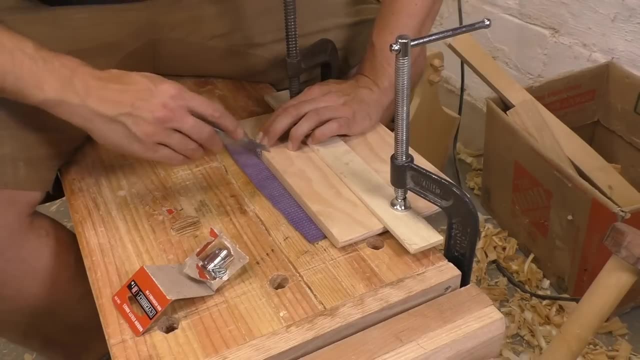 I grabbed these at the big box store and they were under $2 and came with the screws. I will link to something similar down in the description. Place your hinges on the lid an inch or two inches in from either edge and mark them. 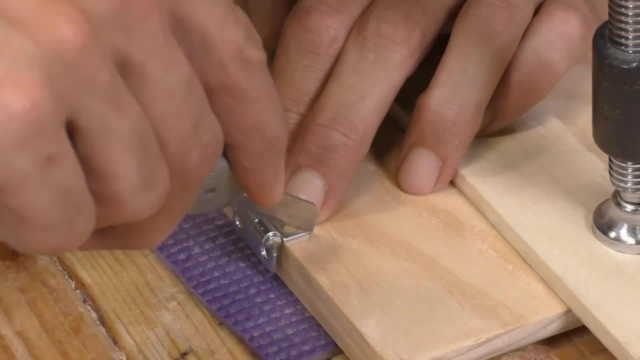 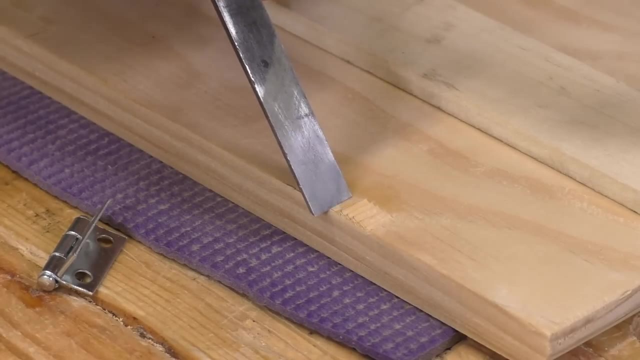 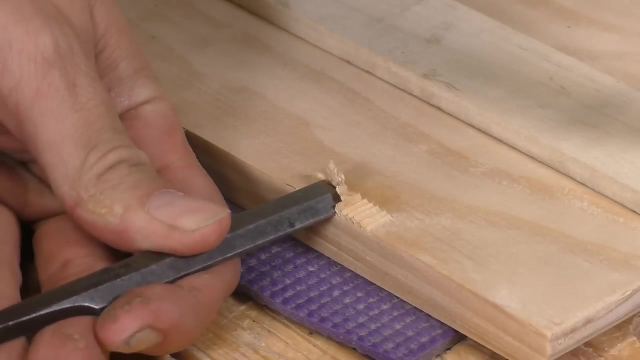 with a knife You want to make several light cuts to get a deep line all the way around the hinge. Then take a chisel bevel down and use light taps across the grain to slowly loosen that waste in chips. Then go in from the side and clean it out with a nice flat bottom. 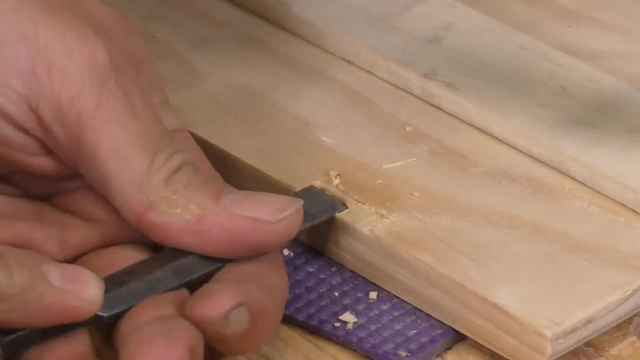 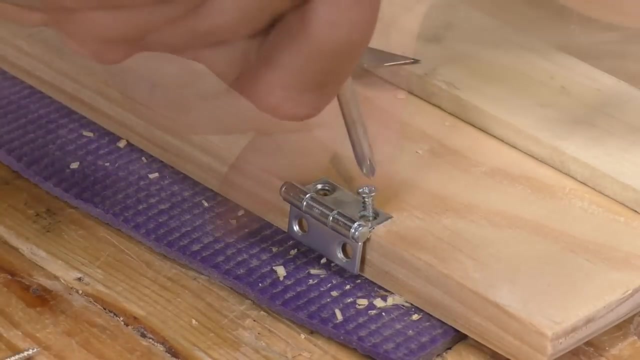 Repeat this process a couple of times until the hinge sits flush with the underside of the lid, Because we're using soft white pine here. you can just prick the screw holes with an awl and run the screws in by hand, Or even better, 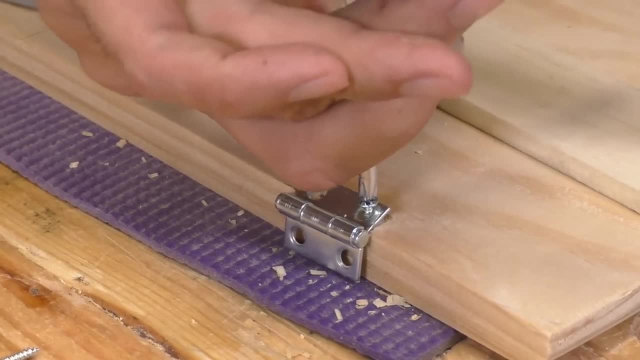 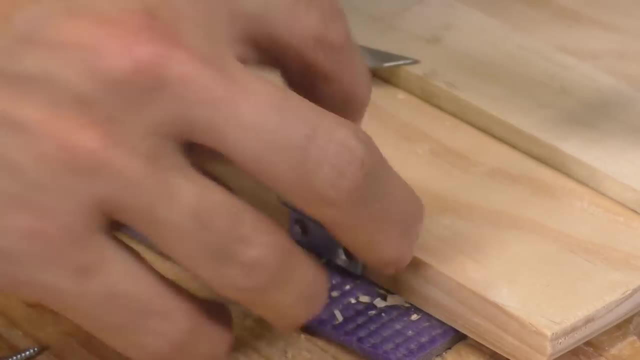 Fill some little pilot holes and put a little bit of wax or bar soap on the threads of your screws. You're going to need to get them out later for finishing and you don't want them stripping. Once everything's cut and clean, you can install your hinges. 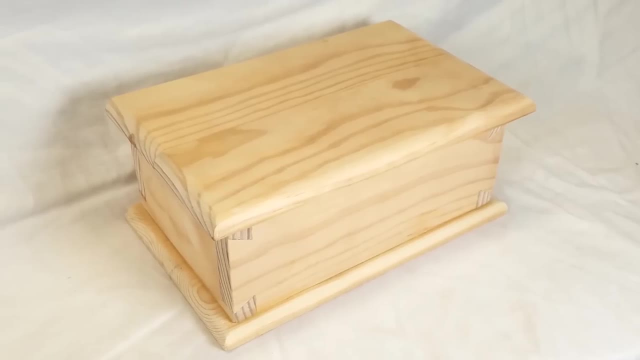 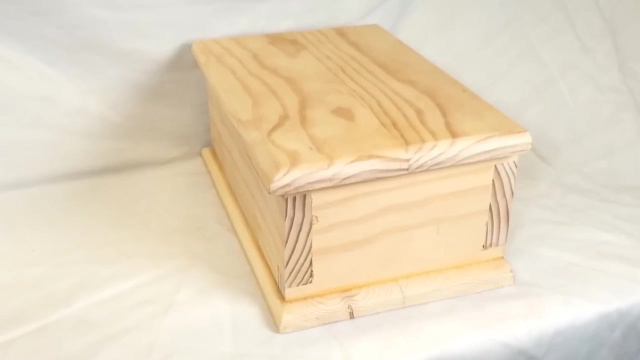 And you know, what started as a simple basic project ended up looking better than expected. It's not perfect, but the whole thing has a nice crisp, organic look to it. It's a lot better than I thought it would be. 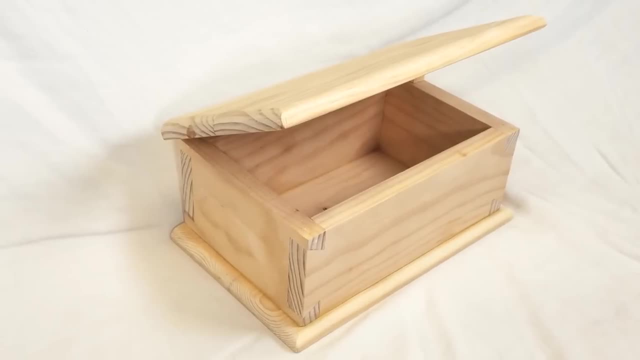 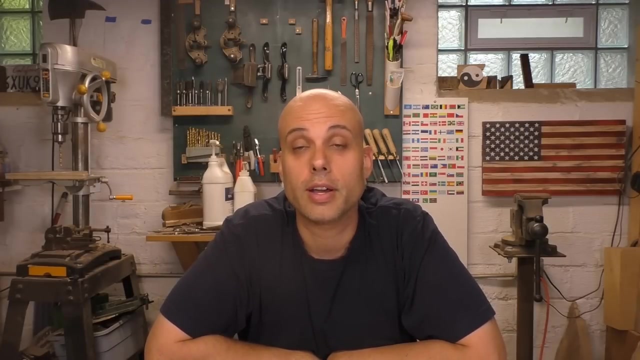 I think it's good enough to give for a gift. I'm probably going to give this to my daughter and I bet she'll love it. I've made a lot of boxes before, but generally with machine tools This is the first one I've done entirely by hand and it is a fantastic skill building. 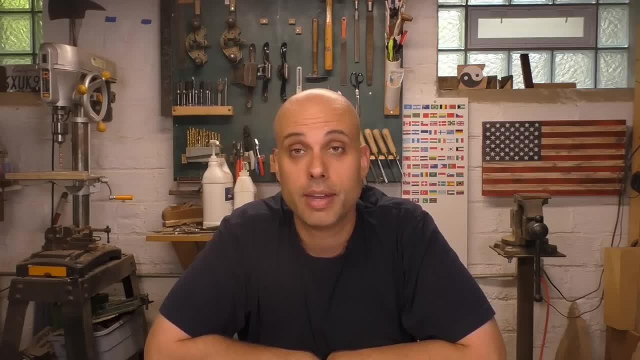 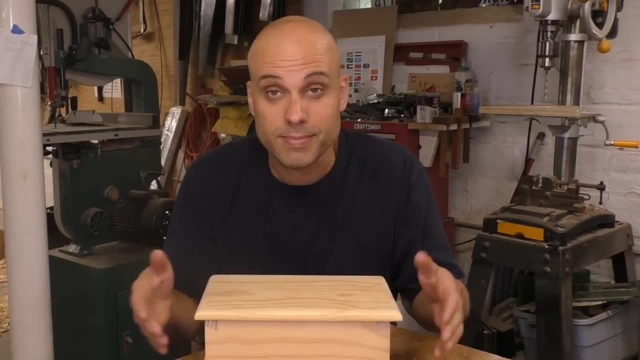 project. If you're even thinking about doing something like this, I recommend you dive into it with no hesitation. It's not very difficult and your skills will go way up from the effort. Now for me, since I finished making this box, I feel like I want to make a bunch more.